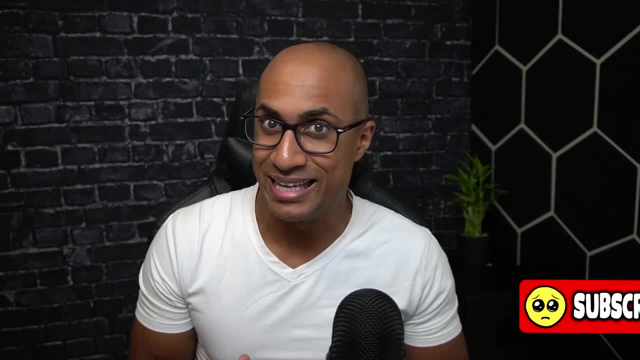 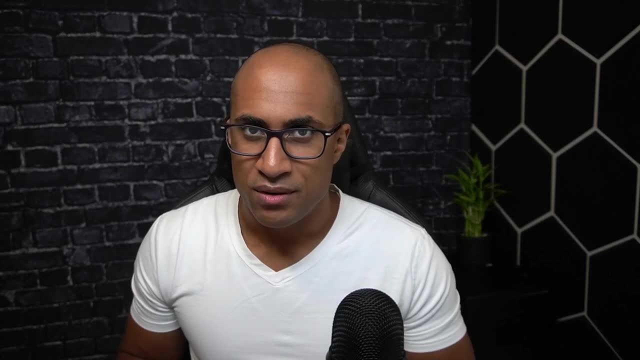 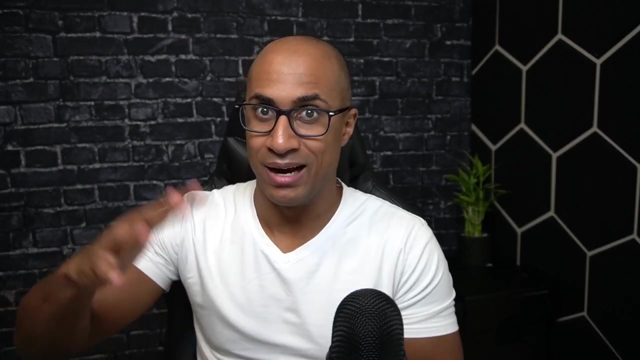 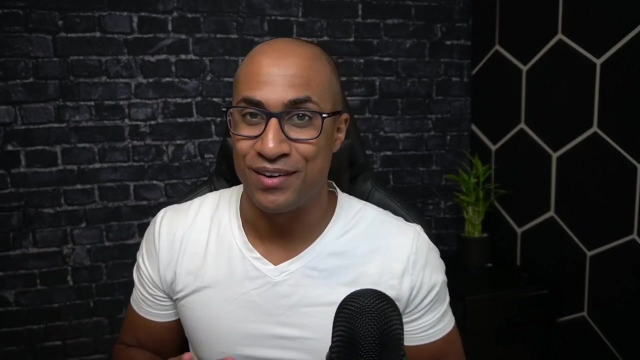 manageable And it's- I won't say it's like easy, but it's definitely like easier than I thought it was going to be. So I'll kind of outline what you can do to kind of take care and do calculus. So in this video, kind of no matter what level your math is, whether it's like arithmetic or like elementary, I'll kind of show you a strategy to like get it up to where it needs to be And then, once it's adequate, I'll show you how to pass calculus from straighterlinecom. So if you're interested in WGU's computer science program, this video is definitely going to be like 100%. 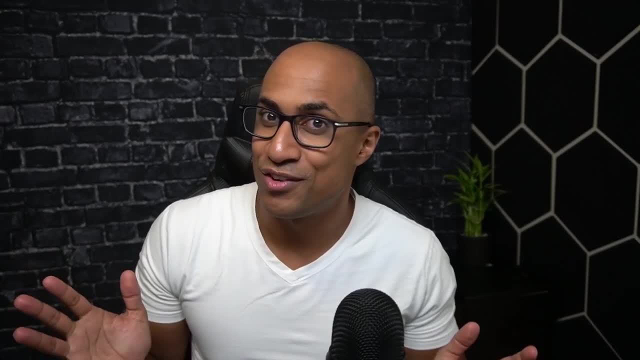 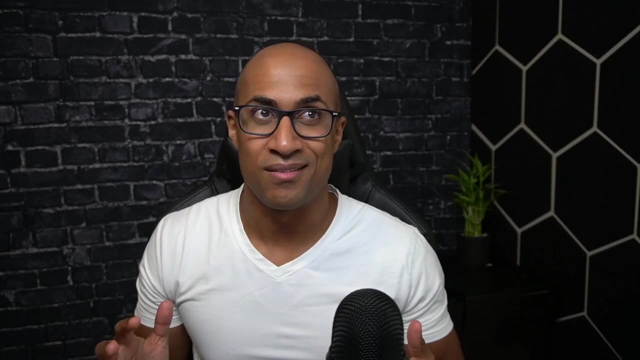 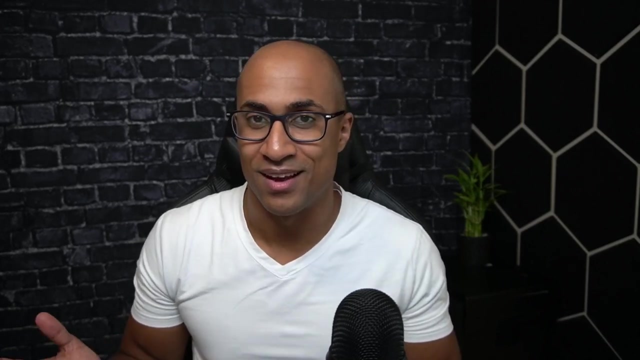 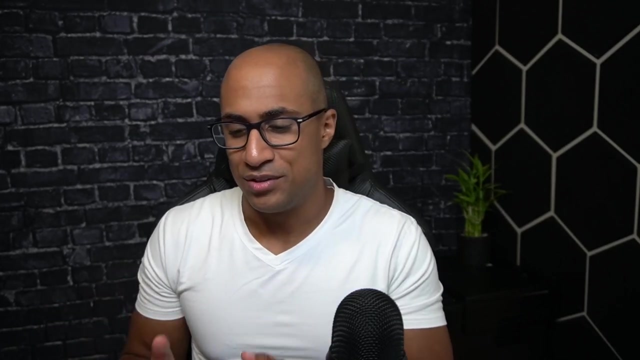 useful to you. So just go ahead and watch the end, like speed it up if you have to, but just watch to the end, it's going to be useful. And for me it's kind of it's hard to say like how long it took, Because, well, just to pass calculus itself was about two months. I could have done it faster, like looking back and kind of realizing hindsight with with my current strategy I could have done it faster. But it's hard to really say how long it took, Because to do calculus you have to be able to do trig and like pre calculus and some geometry and then definitely algebra mainly And like of 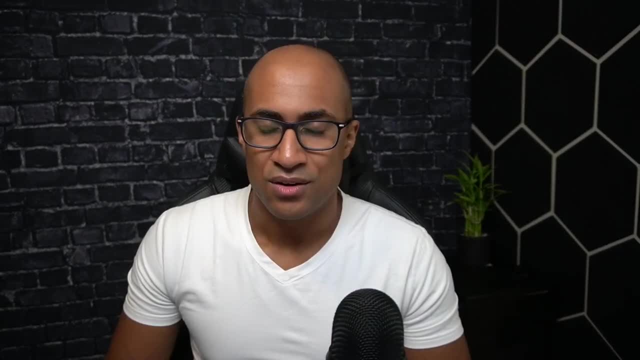 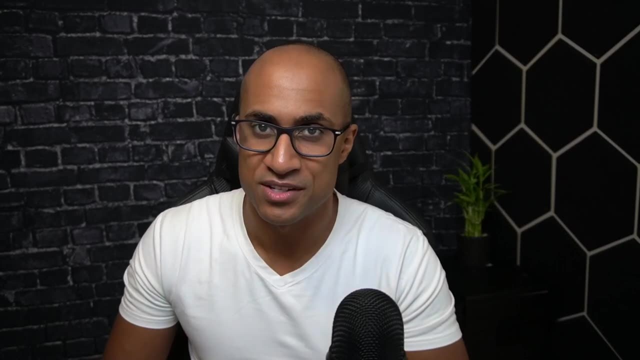 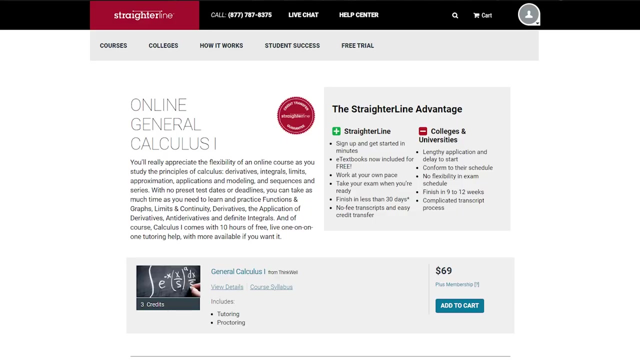 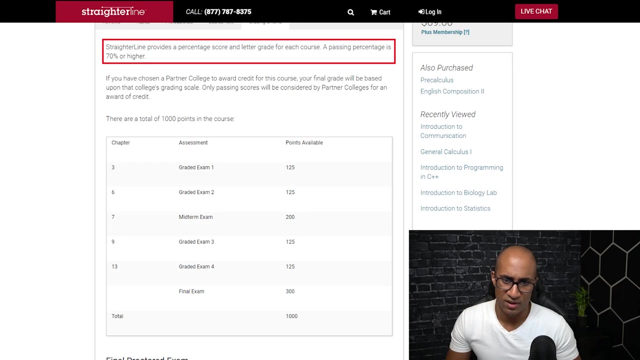 course you have to know how to do like arithmetic and like all those other things. I'll kind of show you how to take care of those in like a really manageable way. But for me, like to calculus itself, it took about two months to do, to be honest. So before I get started on the strategy, let me just talk about straighter line really quick and specifically their calculus course. So this is the page for straighter line, general calculus one. this is a thing that transfers into WGU. So basically this is this is the important part. straighter line provides a percentage score and the letter grade for each course passing percent is 70% or higher. So 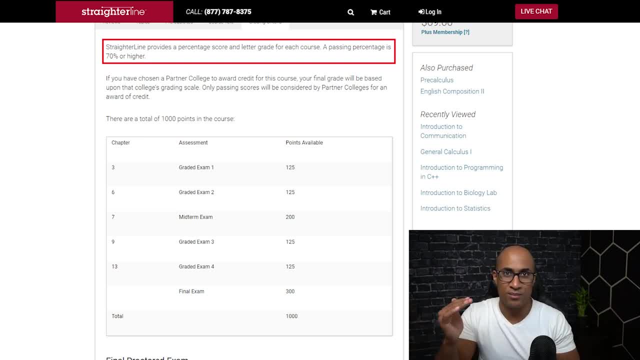 you have to get a 70% on all the curriculum, with all the coursework inside of calculus one to pass. But the good thing about this is basically only some of these are proctored. I believe the midterm is proctored and the final is proctored, I believe So if you can manage, and the graded exams, these are not proctored. So basically you have 1000 points for the whole class and you have to get 700 points to pass. So basically, there's no, there's no reason. I don't 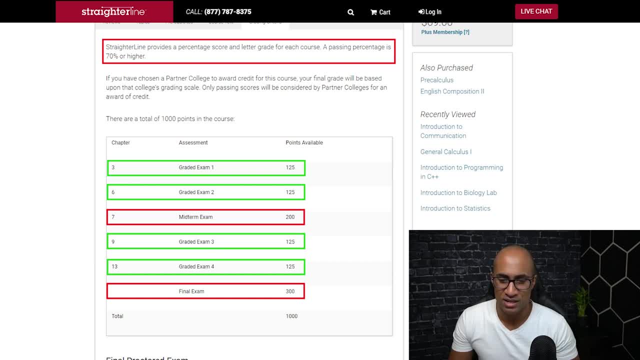 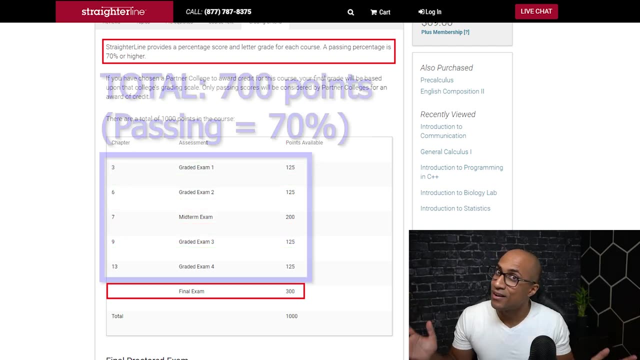 believe, for you to get less than 100% on the graded exams because these are not proctored, they're just like homework. So you can use Desmos calculator, Wolfram alpha, your actual calculator, like whatever, to get 100% on these And then if you can manage to get like close to 100% on the midterm, it means you can just like in theory, right. if you got 100% on all these, you could just not take the final and you'd you'd pass the class without even taking the final, which is proctored. So like in reality, like what your kind of goal or objective is to do is to essentially 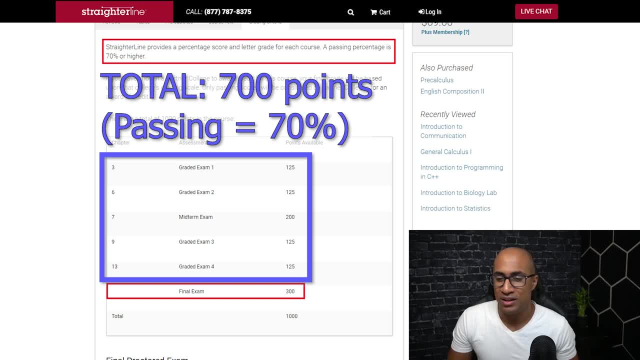 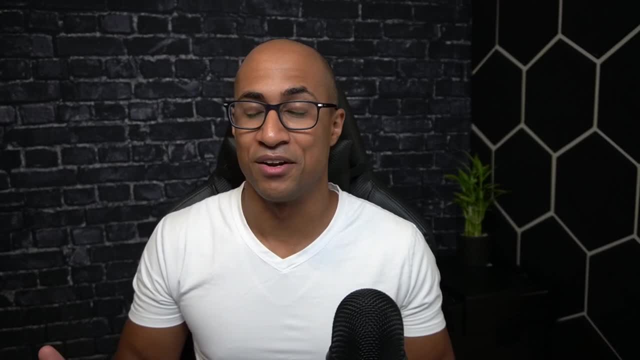 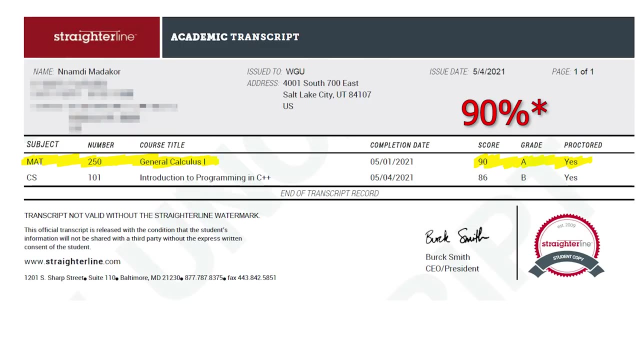 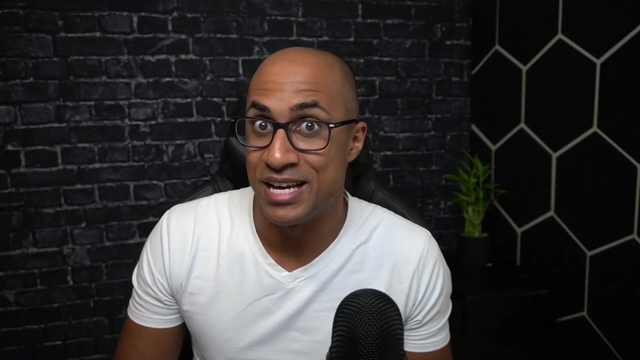 like get 100% on all the homework and then do as well as you can on the midterm, And then you can basically bomb the final and you can still pass in and, you know, get your calculus credit. That's kind of the mindset I went into it And I believe actually I ended up getting like 91% for the whole course because I did really well on the graded exams, obviously because they're not, you know, they're not proctored and you can just, you know, take your time with them and use all the tools you want. And then the midterm I just like kind of did my best on and then I 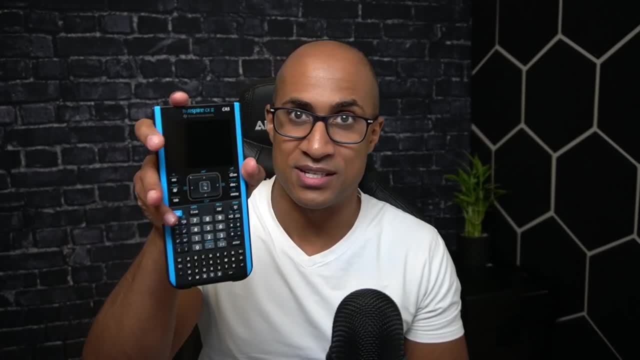 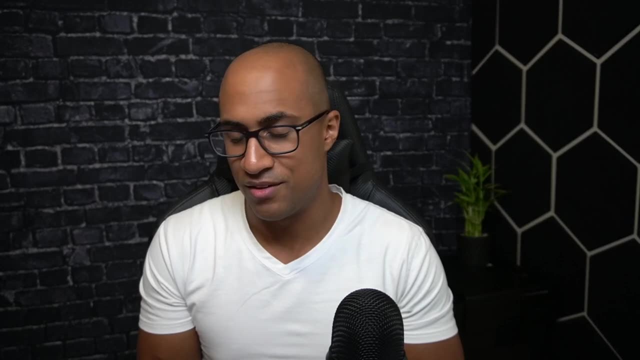 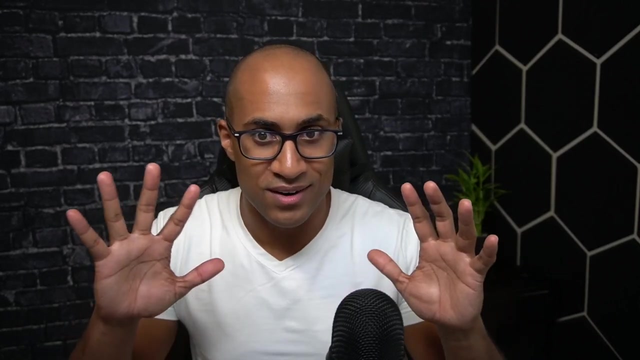 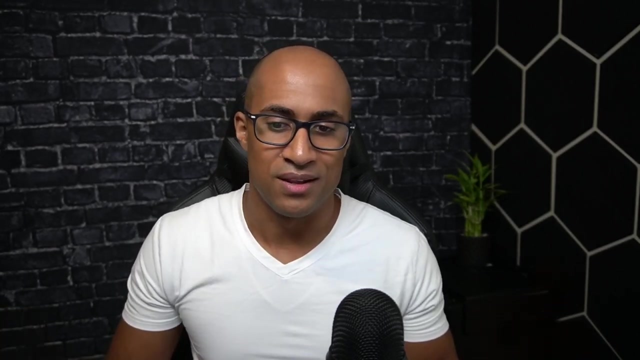 did like okay on it. And then the final. I got really good at using this calculator, which I'll talk about in a second, But I was like really good at using this by the time I took the final- and you're allowed to use this calculator on the final And I just did really well in the final. I got like 91% on the course overall. So yeah, that's just kind- of- I just kind of want to keep that in mind as I'm talking about the strategy- because you know you just need 700 points for the whole course to pass it. you know you get like essentially like free 500 points from the homework And then essentially you can 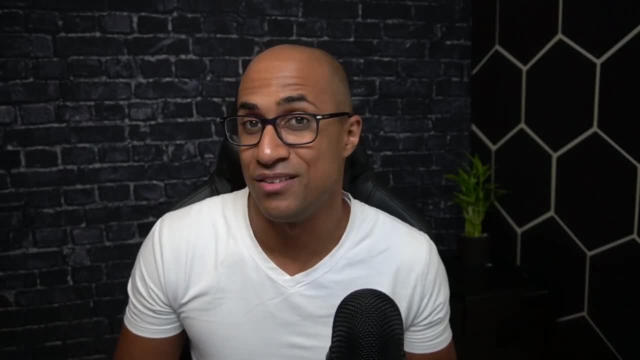 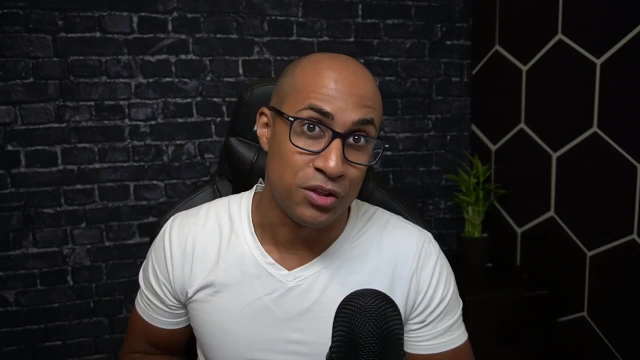 fail both the midterm and final, And theoretically you can pass. you just have to get over 700 points. So yeah, keep that in mind. So, getting into the strategy, if you're serious about this, the first thing I would recommend do like looking back now before you even like kind of realize. 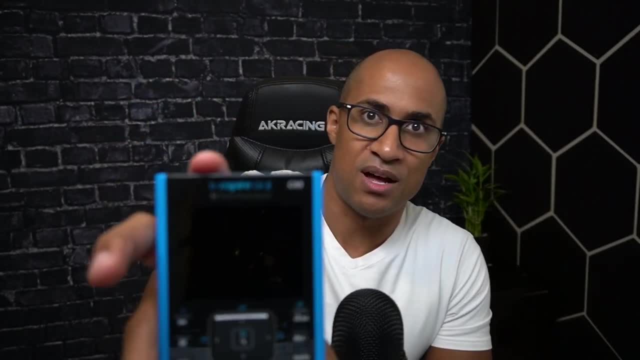 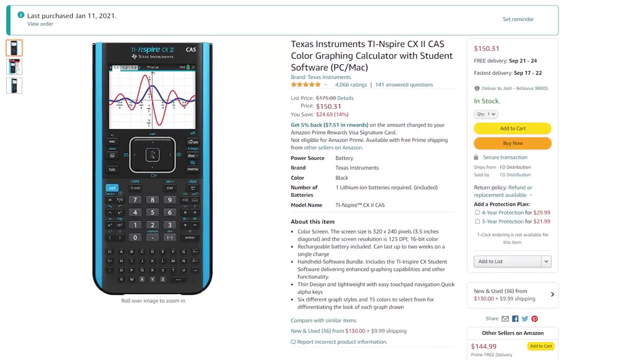 what level of math you are. you should get this calculator. I don't know if you can see it. I'll put a link in the description. I have a feeling it's not going to focus, But this is the TI Inspire CX2 CAS. It's a really fancy calculator And it lets you do really difficult. 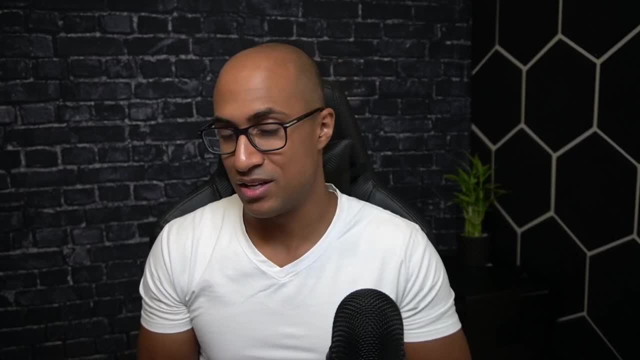 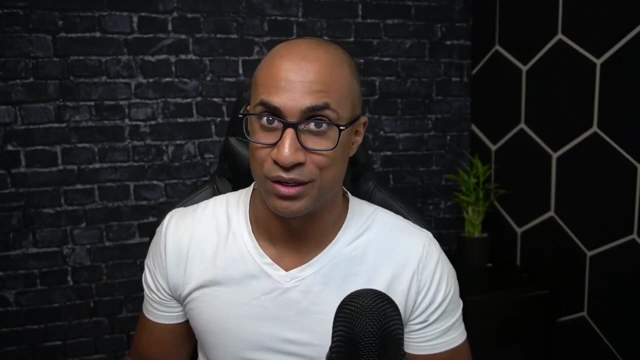 differentials and integrals like really easily. As long as you can do like algebraic kind of gymnastics, it lets you do like the core of calculus computations like really, really simply And it's allowed to use on straight align. So if you want to like go fast and you want to, 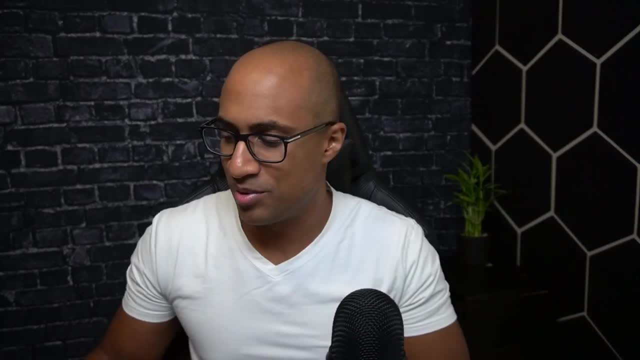 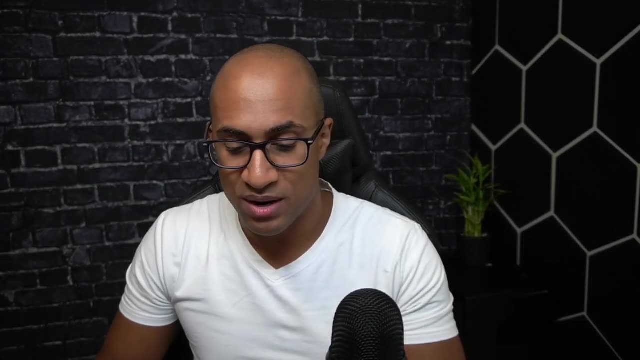 you know, kind of optimize your way through calculus, get this calculator. I'll put a link in the description. So once you have that, you need to kind of figure out like what level your math is right now. So what I would recommend to do is just go to like Khan Academy. So basically, 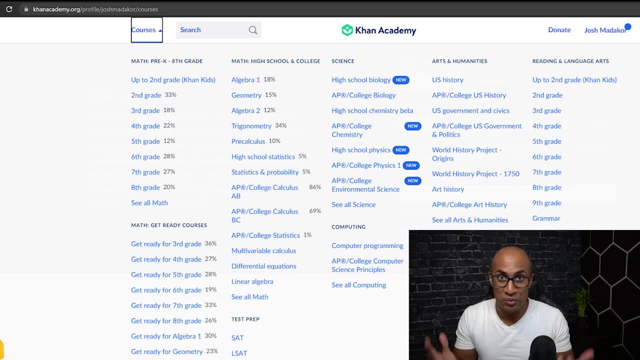 for calculus, the kind of bare minimum, I guess, or what you need to be able to even do calculus. you need to be semi. you know competition, algebra, one geometry, geometry you know for calculating area. like you'll do a lot of weird problems in calculus where you're 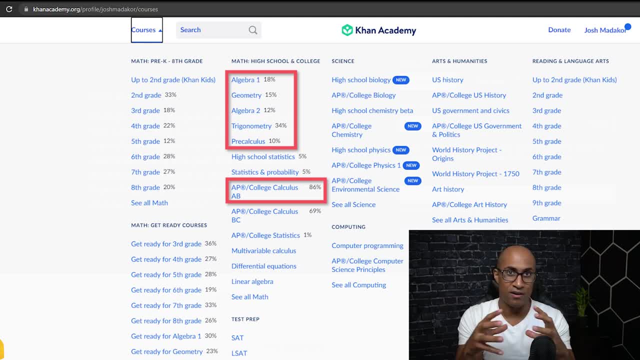 calculating how an area changes, or you're calculating how the volume of, like, a sphere changes, or something like this sounds, sounds intimidating, but don't worry. you need geometry, you need algebra, because that's basically the language of calculus. you need trigonometry. 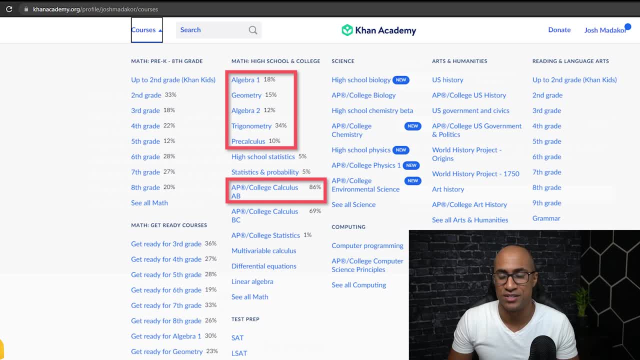 there's like a lot of sine and cosine and triangle type things you have to deal with. there's a lot of like differentiating and integrating trig functions. So you need trigonometry, you need pre calculus. there's going to be like a lot of graphing in here. 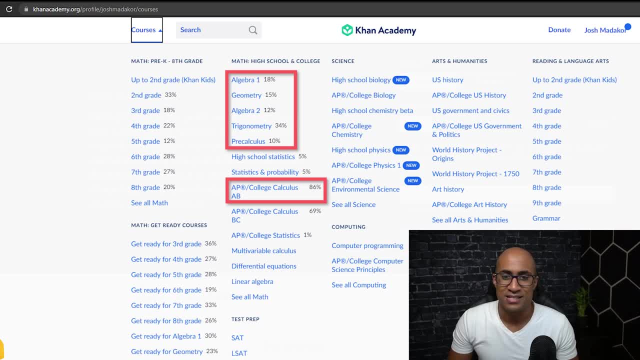 And there's like a lot of graphing and pre calculus. you don't need stats and you don't need probability. you need these two things for discrete math, two and probably one as well, But for this, for calculus, you don't need these. And then the basic, like the objective before you. 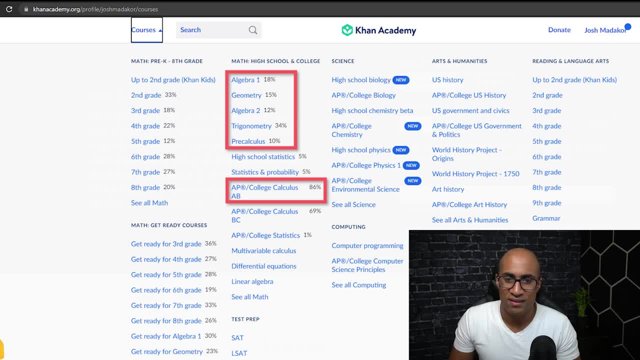 register as straight align is to complete most of this AP calculus. So you need to have a lot of calculus AB course here in Khan Academy. So if you don't, if you don't know where you are in math, I would honestly just pick like algebra one, because I think you only need arithmetic to be. 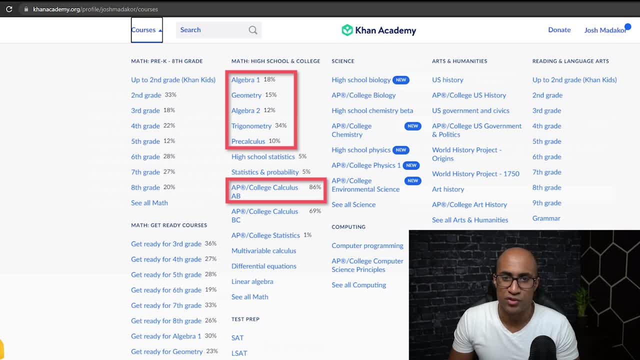 able to do algebra one work through, like all of algebra, one work through geometry, you know if you're if you need to start at trig, start at trig and go through it, But basically just work through these like one at a time, skip statistics and then work through all of this. 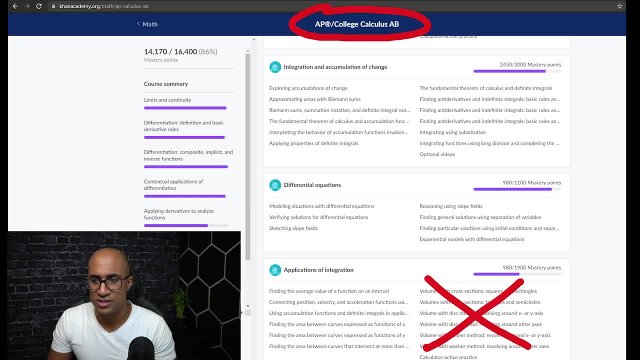 AP, college calculus, AB, except for you don't need to do these volume. you need to do these volume problems. application of integration is useful and it's going to be used on the test, but not the volume. like you know, integrating like 3d things you don't need. 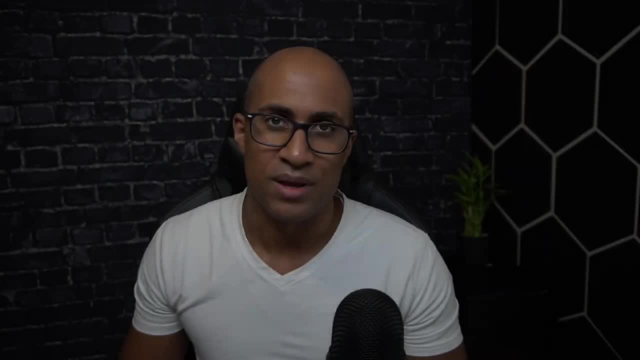 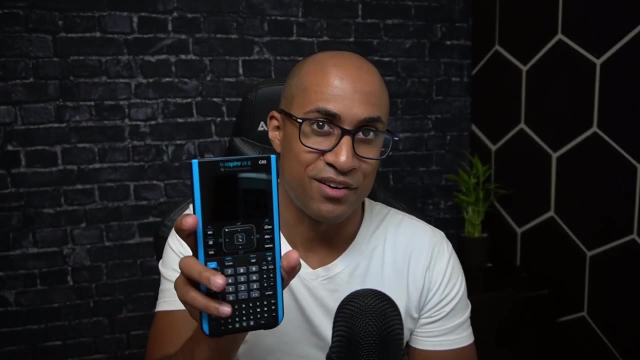 to do that first, straight align. So how I would go through, how I'd go about Khan Academy: just start where you need to start. say, for example, that you're going to start in algebra one. like you already have this calculator because you bought it And the whole purpose of this is to 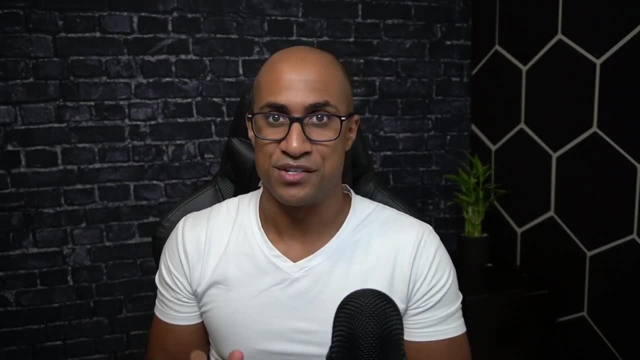 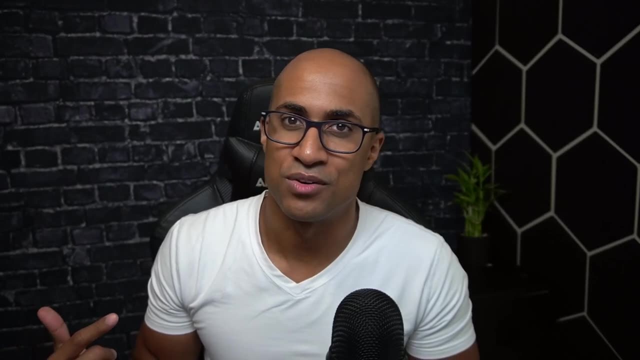 kind of get used to using it So you can get like really efficient at using it. So I would do algebra through it and Khan Academy. you don't have to get like 100% on everything. Don't waste your time doing that you know. settle for like 80% If you like. miss a problem here and there, don't don't. 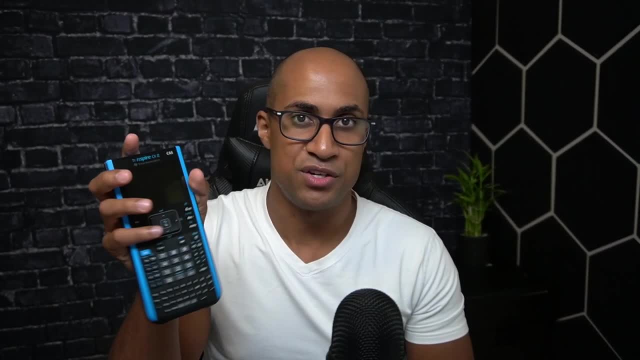 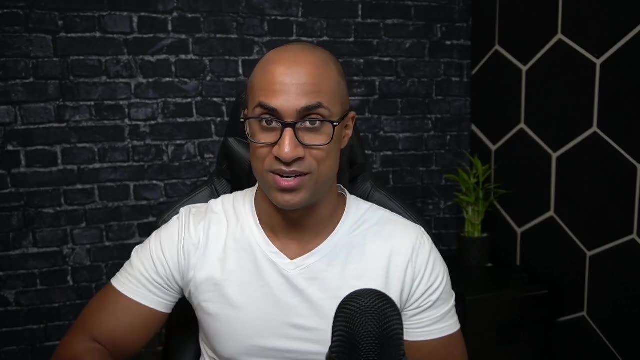 get mad and try to get 100%, But wherever it makes sense, kind of use your calculator to work through the problems. I didn't do this. I didn't really realize that I could use this And I was using like pen and paper because I wanted to like. it's good to do that Because you know neural pathways. 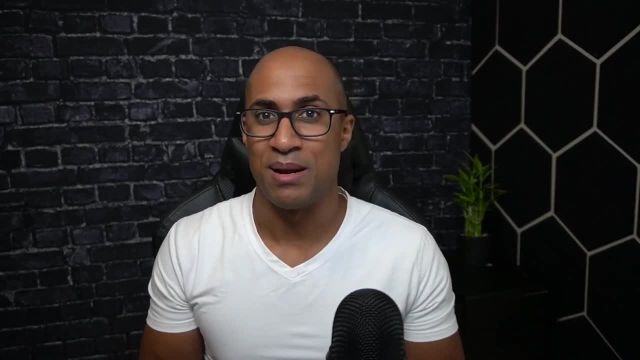 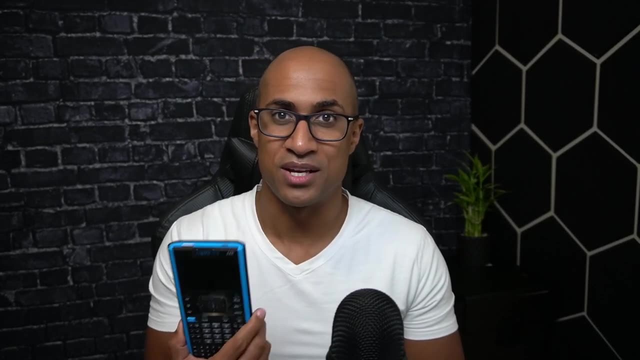 and like all of that stuff. but I use like probably 300 sheets of paper for my like prep on math when I didn't really have to. I could have just used this calculator and got really good at using it and like blaze through like Khan Academy way faster. it just makes you understand what you're doing, But you know work. 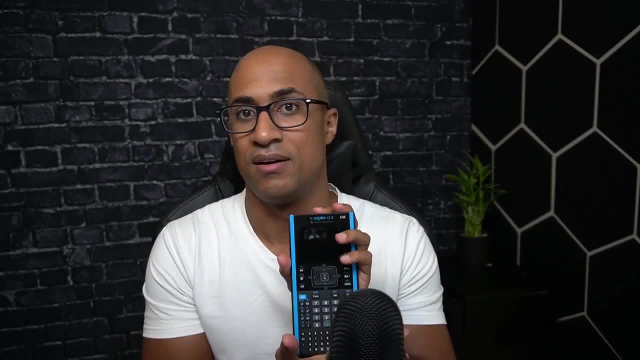 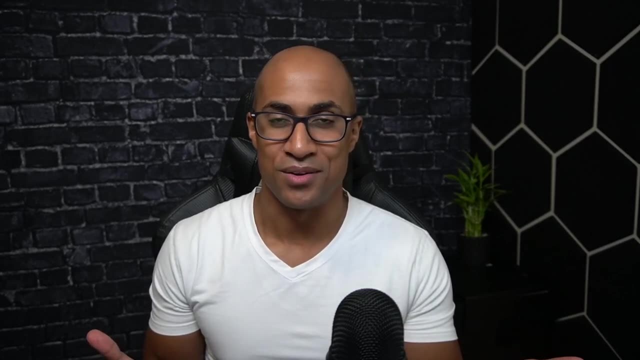 through all the required things at Khan Academy and kind of use this calculator as you go And especially gets useful, like when you get into the calculus section. you know, don't get mad and too frustrated you can. you know, use Reddit and ask people questions and like think hard and like use. 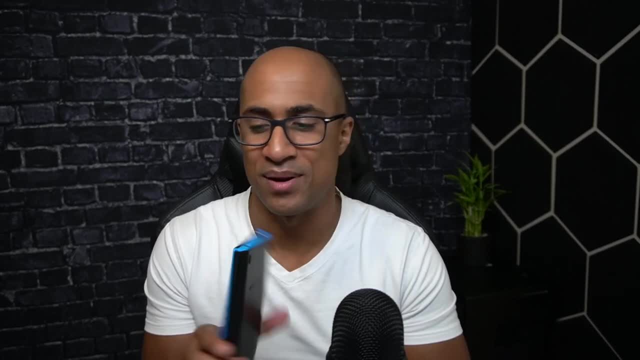 your calculator. just make sure you know, like, what you're doing and what's like happening, because this calculator is like super useful come time for the exam. So once you've kind of worked through all of the Khan Academy, you're going to be able to use this calculator to do all of your. 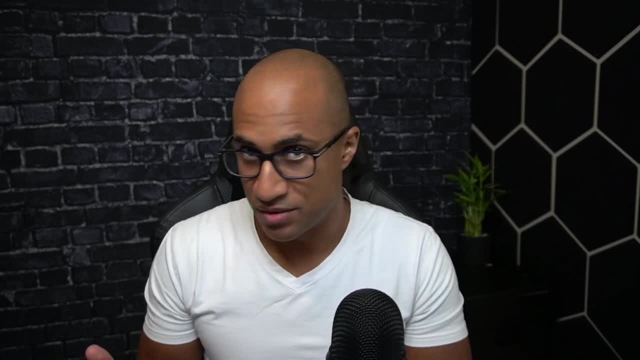 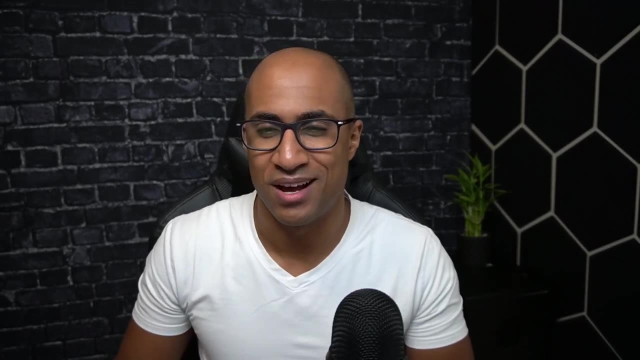 math and you finish the AP calculus a B course and minus the volume part, Now you can go ahead and register at straighter linecom. Make sure you're registering for the right class. It's like general calculus one, So once you're registered, just kind of work through all the curriculum. 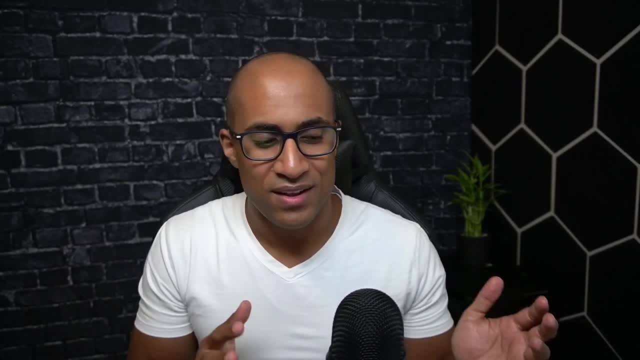 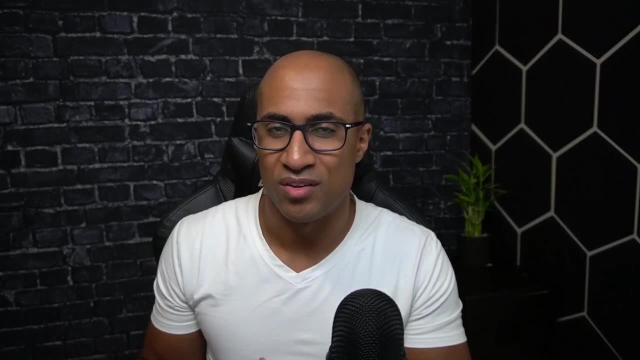 are all the problems I gave you just to kind of get a feeling. it's kind of like when you go from one math teacher to another you're kind of thrown off guard sometimes because different people kind of give you different kind of problems a little bit, And I know I noticed a straighter line problem. 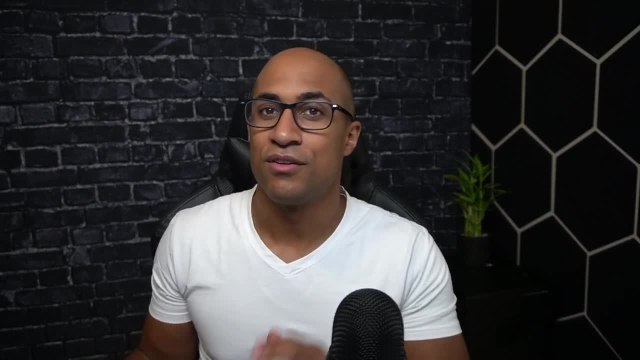 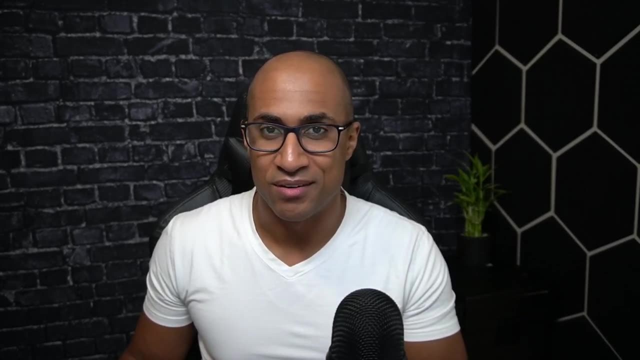 So it's still calculus, but they're like a little bit different. So just take your trust calculator right and go through all the homework, watch the videos if you need to, to kind of get a, to get that straighter line flavor. I guess you can watch the videos there. 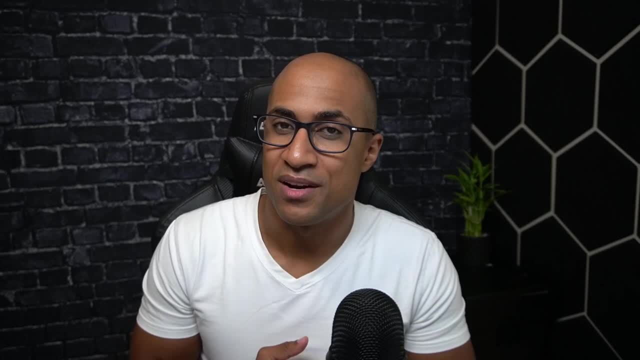 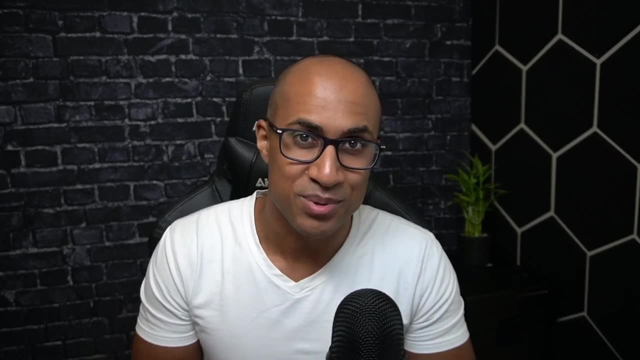 but go through all the problems when you're doing the exams. try to get 100% of those because they're not proctored And it's going to like help you a lot when you need that 700 points to pass the class. So get 100% on all the graded exams By the time you do the midterm. you'll be like really. 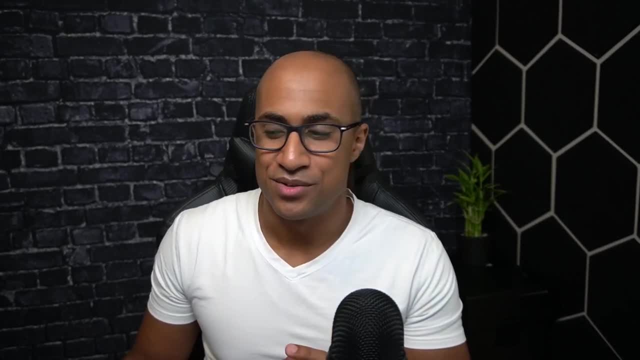 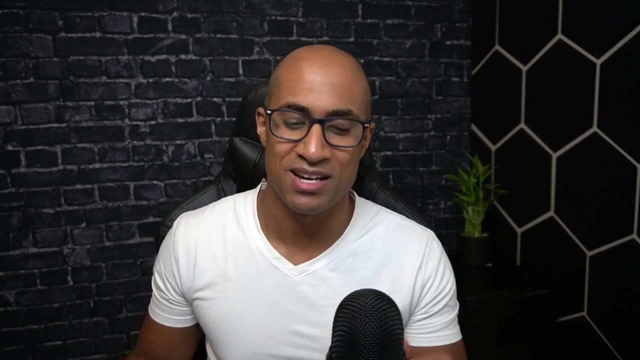 good at using this calculator and just do your best on it. right use- you know you'll have been differentiation and stuff on this. it's going to be like kind of- I don't want to say cakewalk, but it's going to be like kind of kind of easier than than one might expect. So do your best on the. 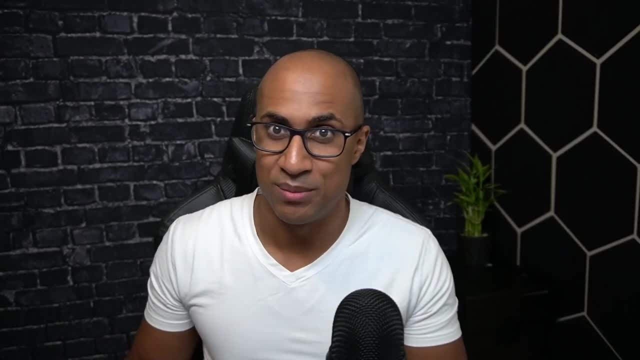 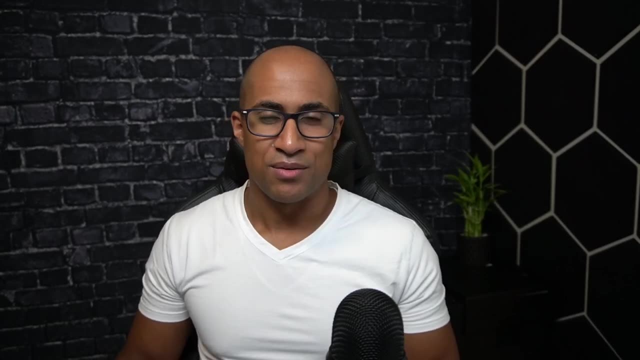 midterm And you know, do your best on the final gear calculator, just do your best in the final and then you're- you're simply going to pass the class at this point. So that's, that's pretty much all there is to it. Some kind of pointers and pitfalls that I would recommend to avoid is: don't. 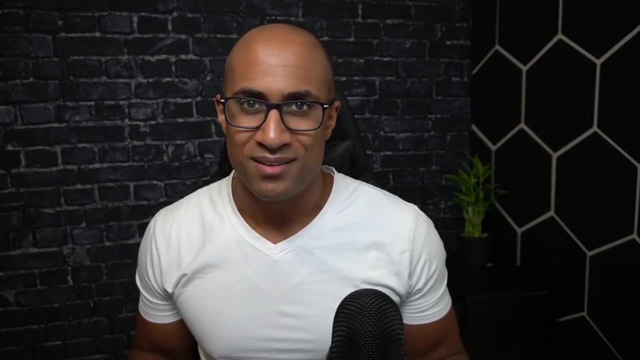 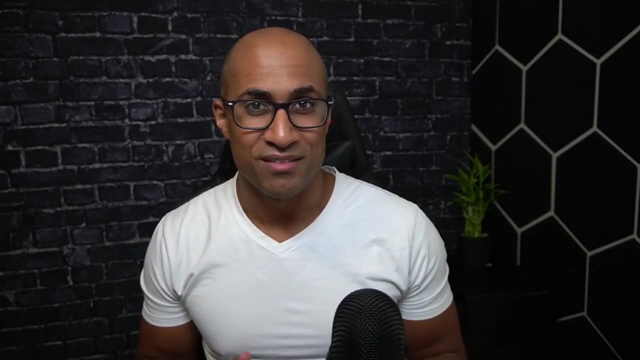 work on math like too much per day. it's going to take you a while to do like you can't really. you can't really study math for more than like hours a day before your brain starts like dying. For me it might even be less than two hours And 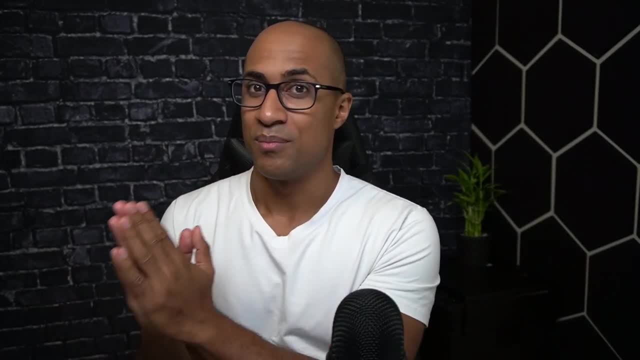 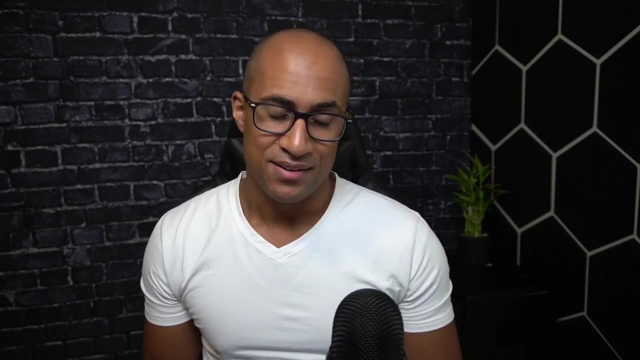 it's kind of frustrating because you have more time and you want to do more, but it will really burn you out like quick if you're doing math like eight hours a day and you'll you'll not be able to finish it. This happened to me, honestly, when I was trying to do it, I had to take a break for. 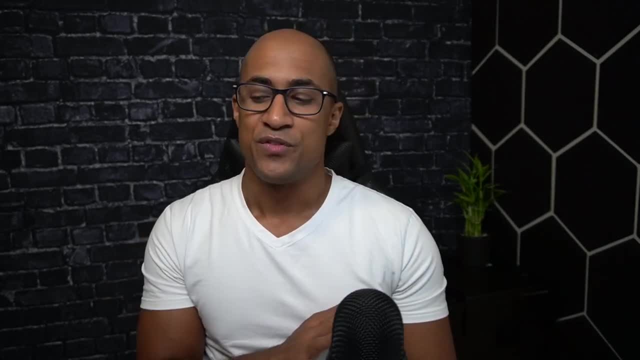 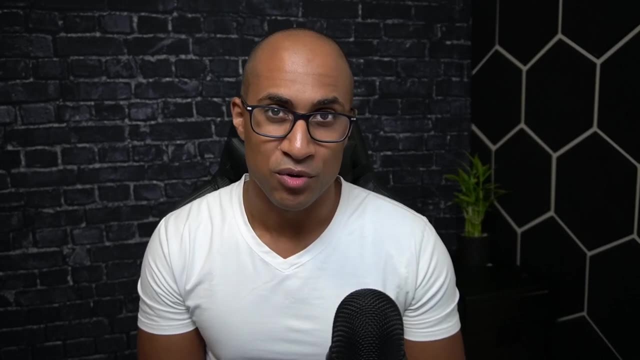 like a month because I like overloaded my brain. So don't do this. just get your calculator and work as you're working through Khan Academy. just do like maybe max like two hours a day, And if you feel like you can do more, that's good. But just don't do more and go watch Netflix or do something. 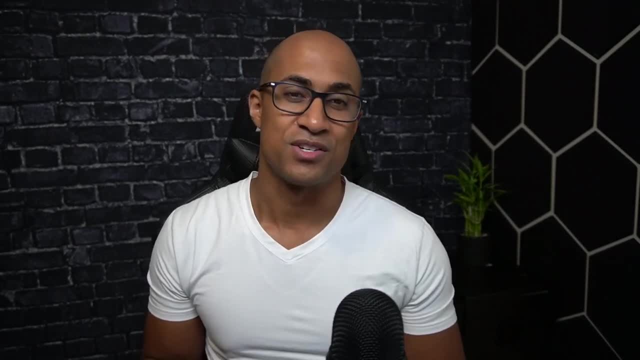 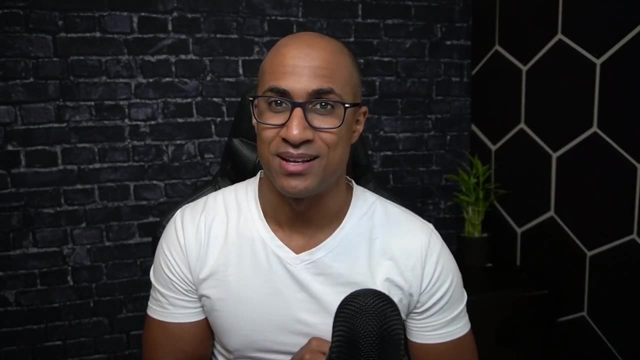 else with your, your poor brain, So don't work too hard on it. First, first, first and foremost. And secondly, try not to get mad, because it's really easy to get mad and like stressed and and just it's going to make you like mentally tired. So if you're like feeling a problem a bunch of times, 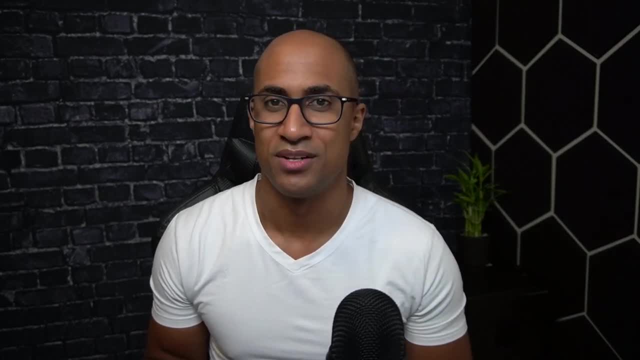 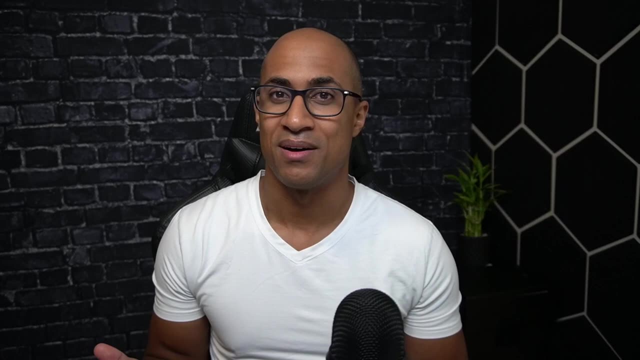 but you feel like you understand the concept. it's okay to like move on to like another problem And if you really want to tackle that one problem, you know, do it, try to do it, but just don't get mad about it because it's not really worth that. like mental energy that you'll you expect, like 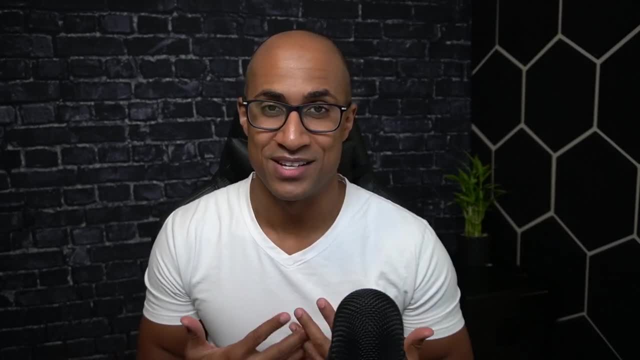 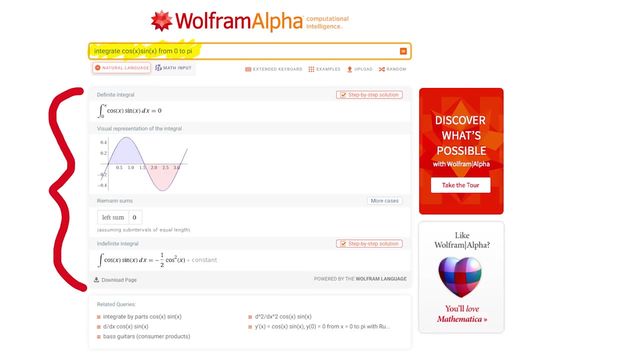 getting really, really frustrated over math, And I'm guilty of this. So that's why I'm telling you to like try to be calm. I guess Another like really useful tip I want to give is use Wolfram alpha, Wolfram alphacom it. you can like plug problems into it And it will kind of like give 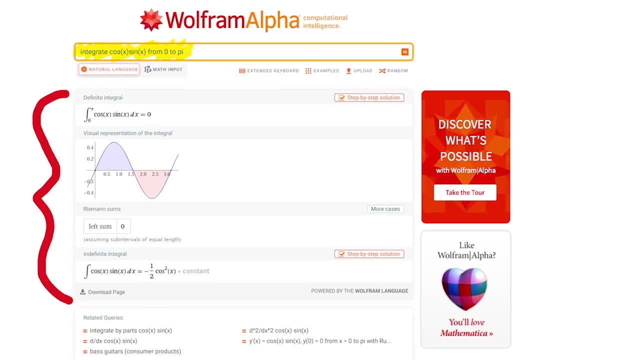 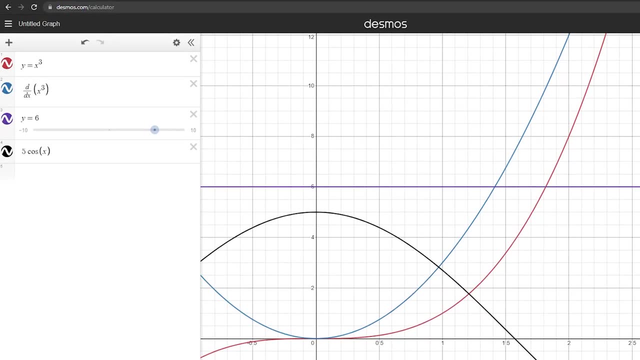 you all the explanation for like how to do different variations of the problem, And it's really useful. I'd also use the desk Desmos- I don't know how, if that's how I'm saying it correctly, But the desk most graphing calculator. this tool is like, also really good. Obviously, use your own. 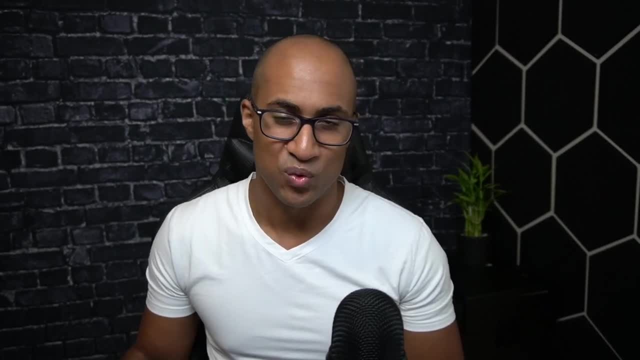 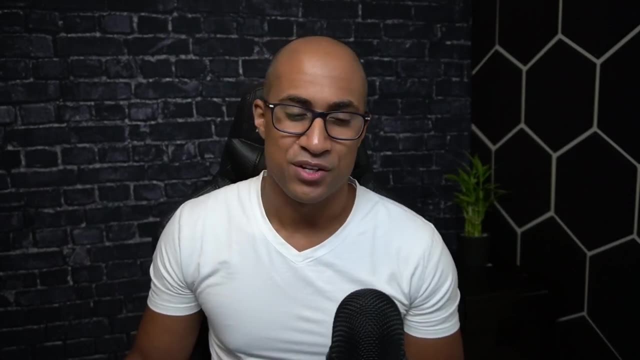 calculator, but the web graphing calculator tends to be like really easy if you just need to like punch in like a quick graph and like see something like quickly, whereas this is like slightly less intuitive. But I use those two things like a lot during my studies, like Wolfram alpha and 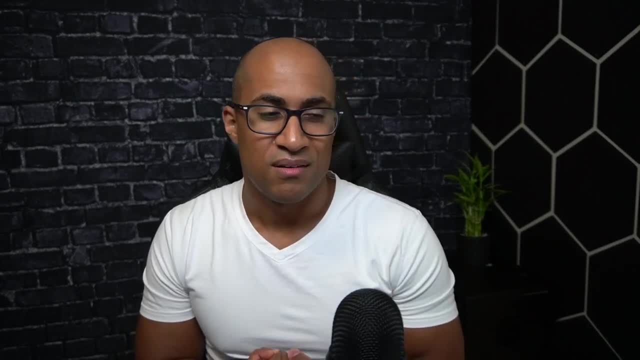 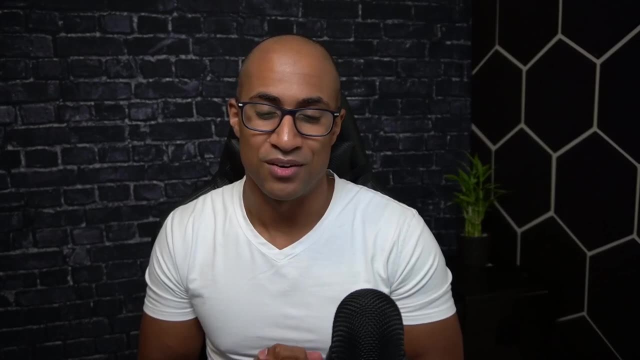 Desmos graphing calculator. So yeah, that's pretty much all I had to talk about. Just enjoy your time and studying math and enjoy conquering calculus. you can definitely. you can definitely, you know, pass it and get the credit transfer into WGU and get your comp sci degree. 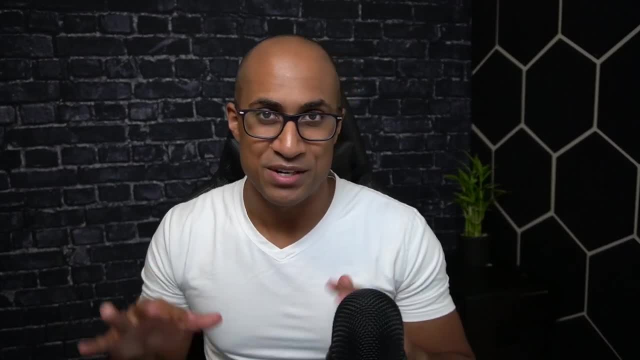 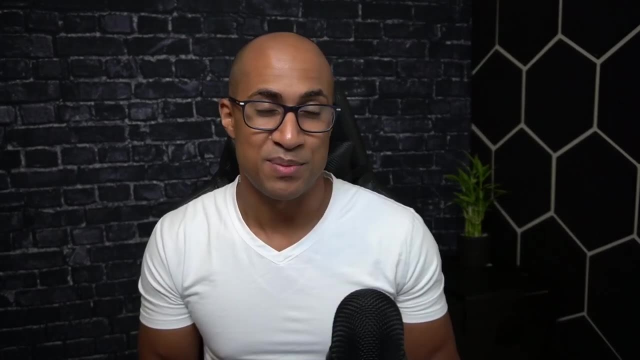 calculus is a big barrier for a lot of people, but it doesn't have to be, especially with this kind of setup, in this strategy, And like all the tools at your disposal it's. it's much, much more manageable these days, especially with this kind of strategy that I laid out here. So again, I'll put a link to: 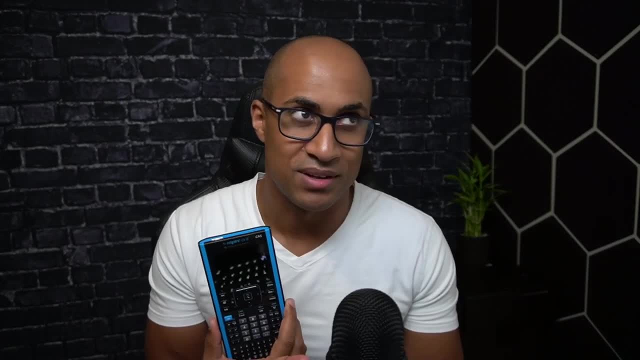 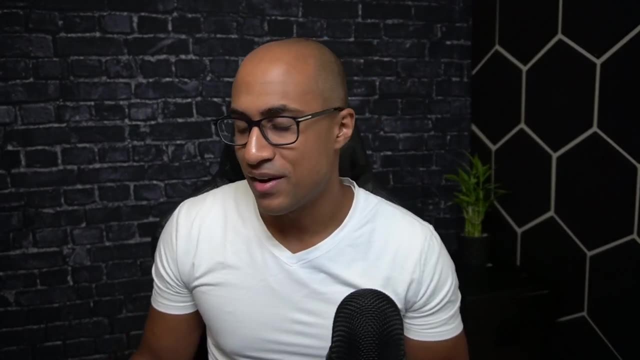 the calculator in the description It's an affiliate link, So I'll get money right if you use it. if you don't believe in affiliate links, you know, just look on your own or look, look on eBay or something. I tried to find this calculator. 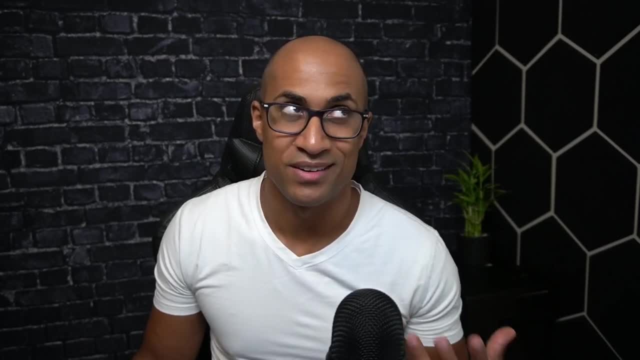 on Craigslist but it's like super hard to find And I tried to find it on eBay. it was either hard to find or the price was like the same as a new one, So I just ended up buying it on Amazon. So I